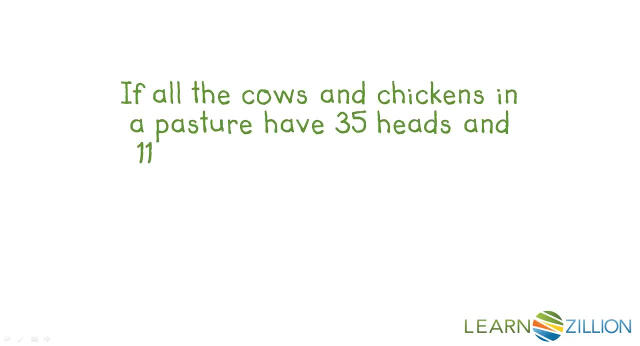 If all the cows and chickens in a pasture have 35 heads and 110 legs, how can you use a system of equations to help you find the number of cows in the pasture? In this lesson, you will learn how a system of linear equations can help you model a real 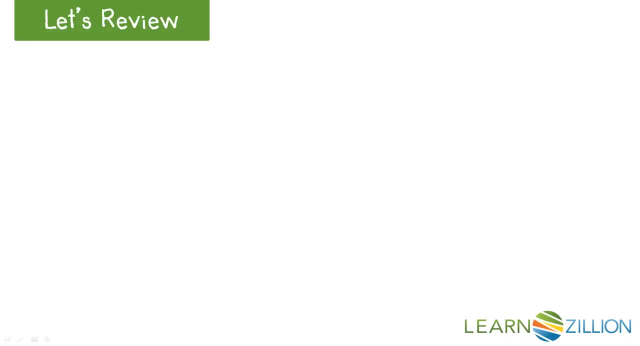 life situation by analyzing a problem. Let's review the important vocabulary. A system of equations is a set of two or more equations with the same set of unknown values which are represented by the same variables. They are also called simultaneous equations. Here is an example of what a system of equations. 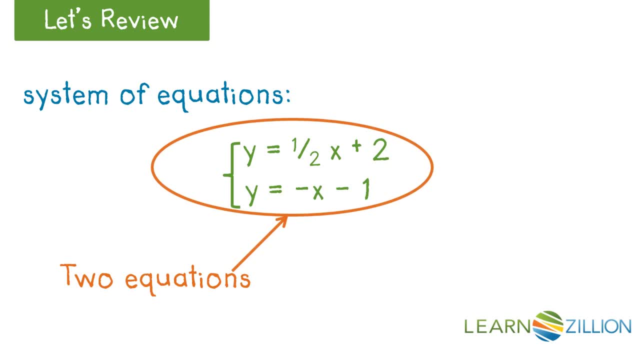 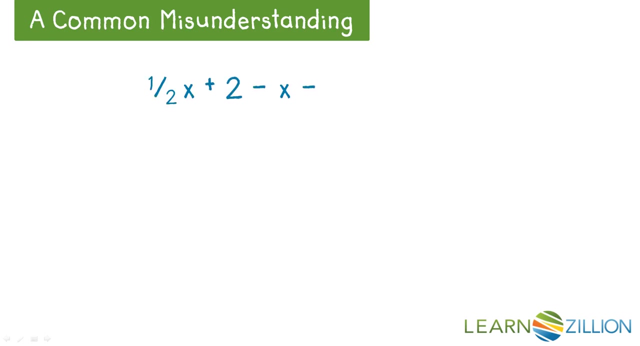 looks like. Notice that both equations have the same two variables, x and y. The brace on the left is written to show that the equations are simultaneous. That is, the variables x and y represent the same unknowns in both equations. A common misunderstanding is the idea that all of the information from a problem should. 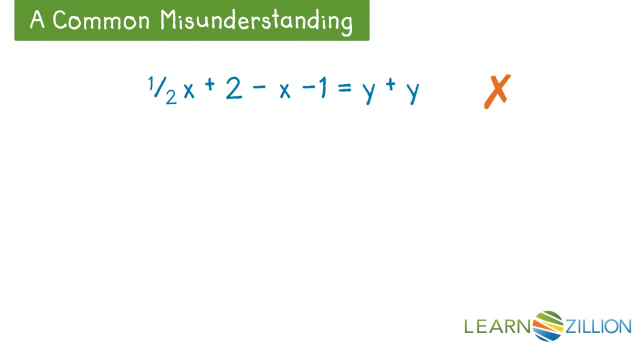 be written as a single equation, While this is sometimes possible for finding a solution. remember you are writing a system which is two or more equations with the same unknown values represented by the same variables. Remember to write a brace on the side to remind. 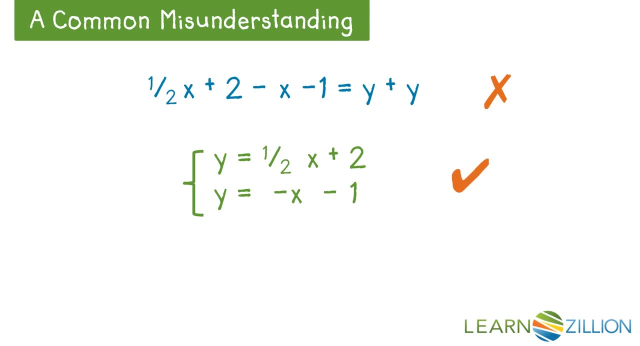 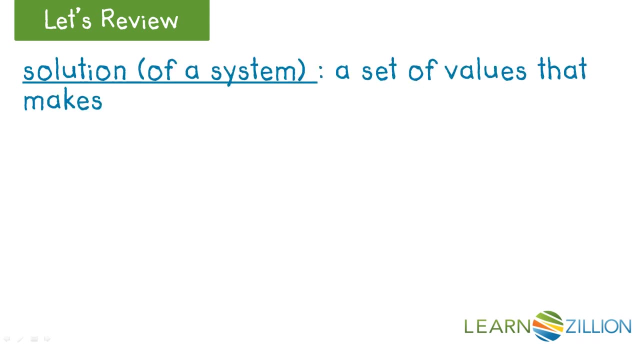 you that the equations are simultaneous, that the variables represent the same unknowns in both equations. The solution of a system of equations is a set of values that makes both equations in the system true at the same time. That means that if we substitute the two equations, we get the same two variables, x and y, The 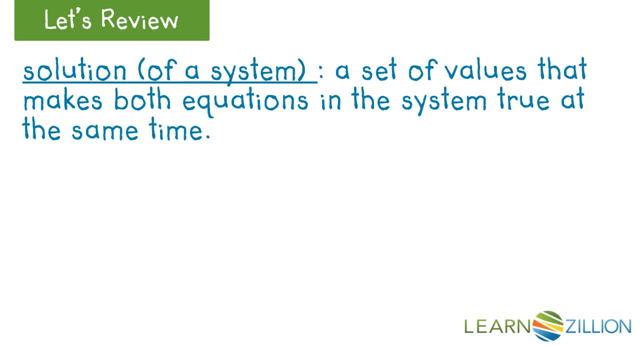 solution of a system of equations is a set of values that makes both equations in the system true at the same time. That means that if we substitute the values in our solution for the variables in the equations in system and work them out, we will get true statements. 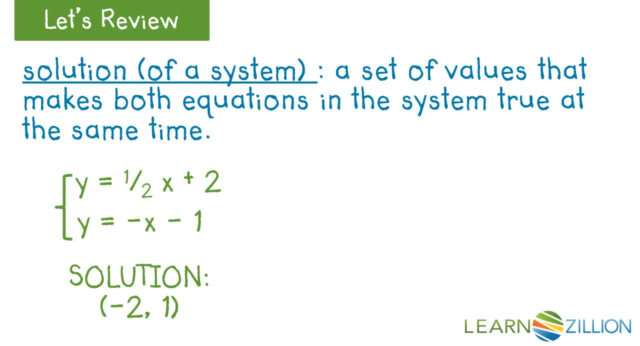 In our example from the last slide, the solution is the ordered pair. If we substitute for x and one for y in the first equation, we get 1 equals 1, half of 2 and 2.. If we multiply the one half by the negative 2, our equation becomes 1 equals 2.. If we 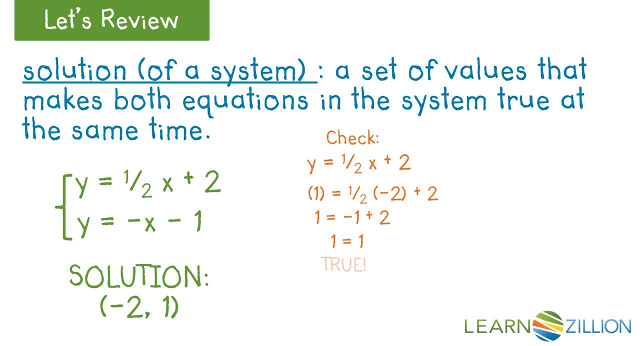 add the numbers on the right, you get 1 equals 1, and, and that is a true statement. The equation of the second line was: y equals negative, x minus 1.. Substituting gives us 1 equals negative, 2 minus 1.. 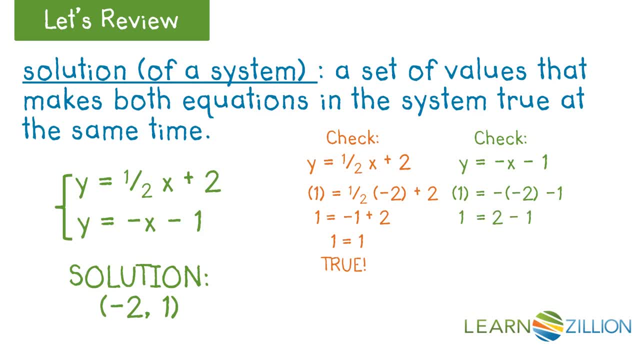 Simplifying gives us 1 equals 2 minus 1.. And subtracting on the right gives us 1 equals 1, which again is a true statement. Notice that any solution for a system of equations must have a value for each of the variables in the system. 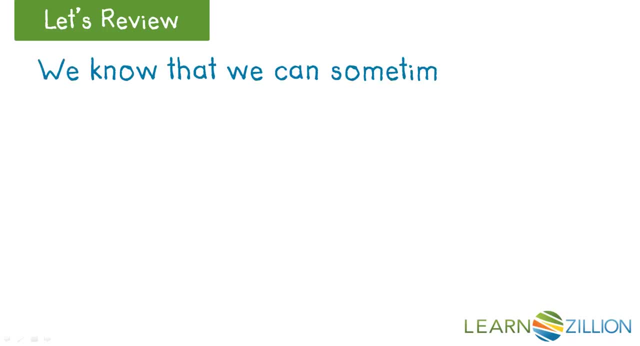 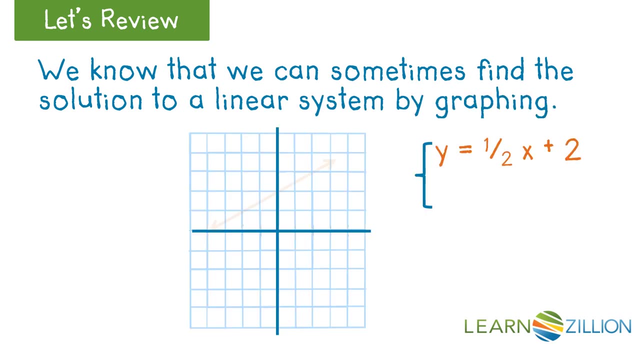 We know that we can sometimes find the solution to a linear system by graphing. Consider our example again. We can graph the two equations in the coordinate system. Their graphs make straight lines and we can spot the solution of this system right away. 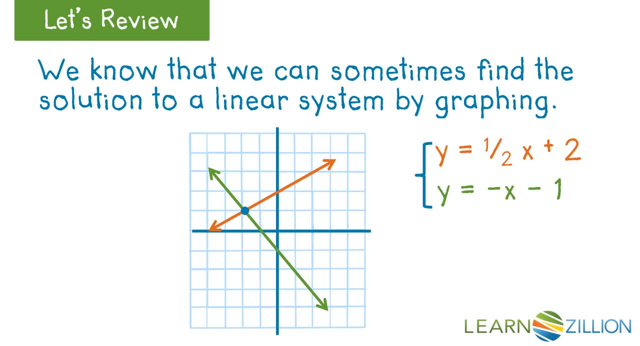 This is because the ordered pair for the point of intersection makes both equations true. at the same time We can see that the lines intersect at the point negative 2, 1, so since the point lies on both lines, it must satisfy both equations. 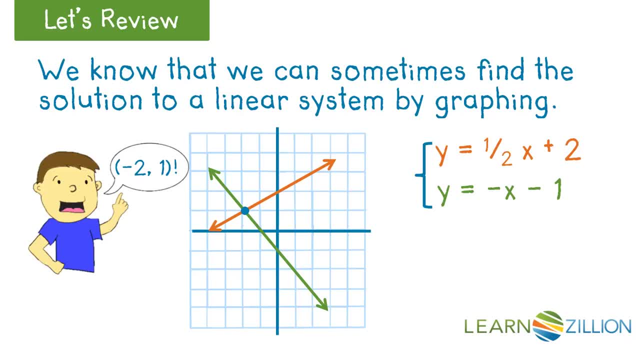 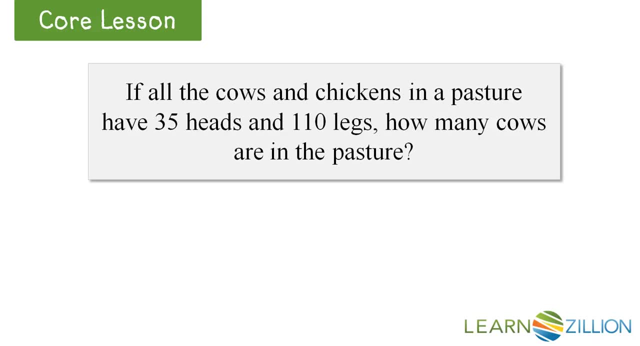 In this way, we can see once more that negative 2, 1 is the solution for this system. Now that we have some introductory information, let's look at a problem that can be modeled using a linear system. If all the cows and chickens in a pasture have 35 heads and 110 legs, 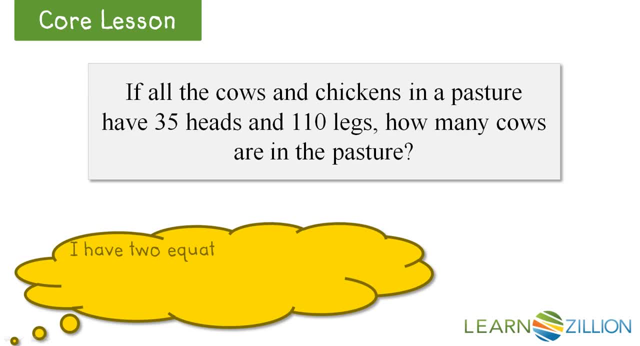 how many cows are in the pasture. We have enough information to write two equations with the same two unknown values and we can represent them with the same variables in both equations. So let's write a system To begin writing appropriate equations for any system. 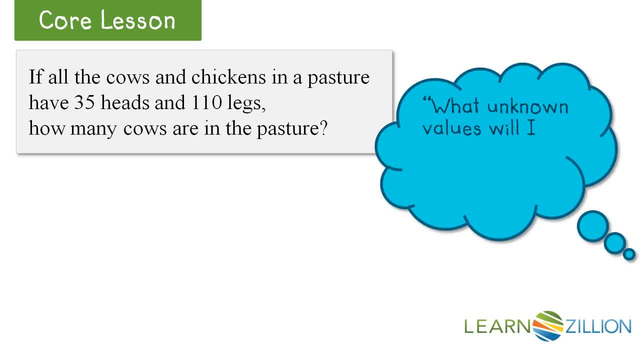 you must first define your variables. So you ask yourself, what unknown values will I need to find for this system And then choose variables to represent those unknown values. This problem asks you about the number of cows, but that's not the only unknown in this system. 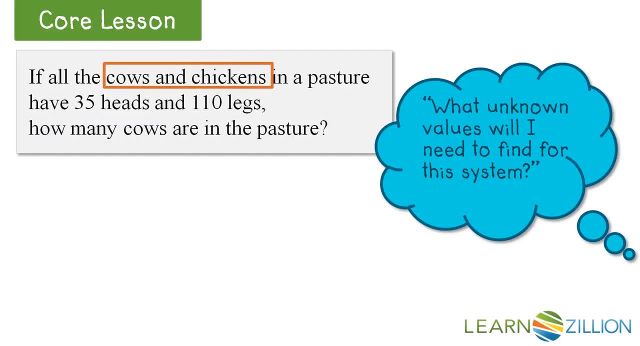 Here the unknown number of cows is connected to an unknown number of chickens, so both of those values must be represented with variables. We can use whatever variables we want, but systems of equations are often connected to graphs in the coordinate system. So let's use x for the number of cows and y for the number of chickens. 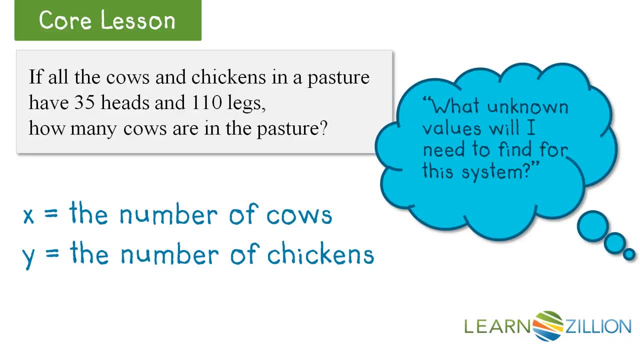 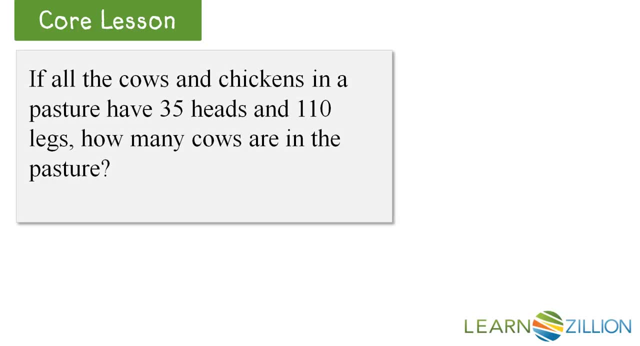 Remember you'll use the same variables for cows and chickens in both equations. Next, examine the problem to see what types of information you have. This will help you write equations for your system. Keep in mind that a system is two or more equations about the same unknown values. 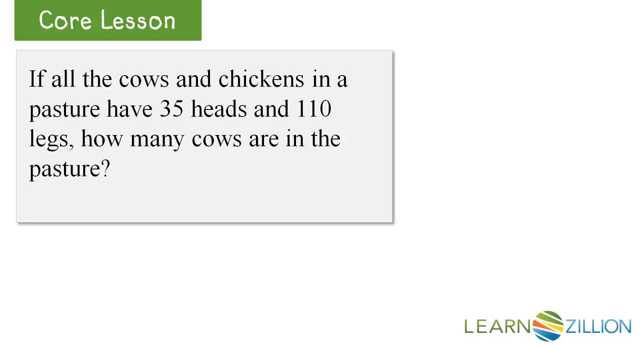 so only the variables used in your equations must represent cows and chickens. This example tells us that 35 is the number of cows and chickens, and the number of chickens is the number of cows and chickens, And the number of cows and chickens is the number of heads the animals have all together. 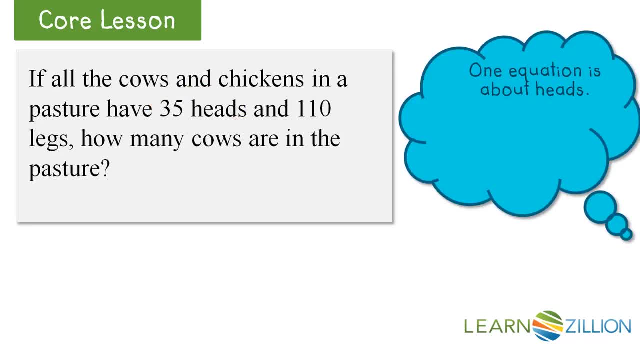 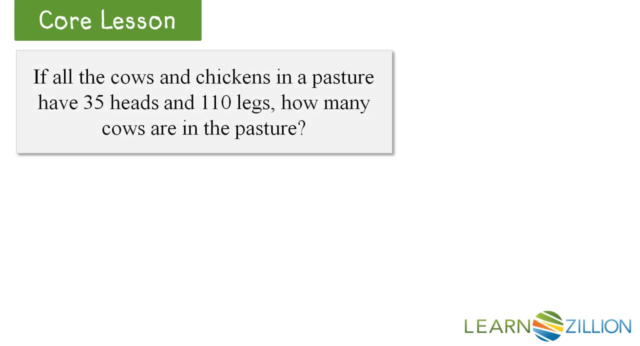 So one equation must be about their heads. The problem also tells us that both groups of animals have 110 legs total, So the other equation must be about how many legs the animals have. Finally, find ideas or words that tell specific numbers and operations to connect. 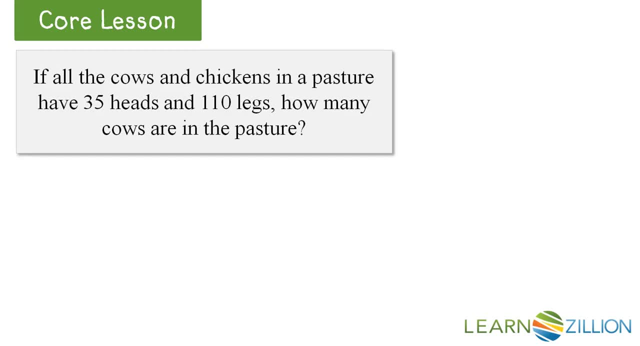 to the unknown values and use that information to write your system. Remember, in step one we said that x was the number of cows and y was the number of chickens. In step two, we said that x was the number of cows and y was the number of chickens. 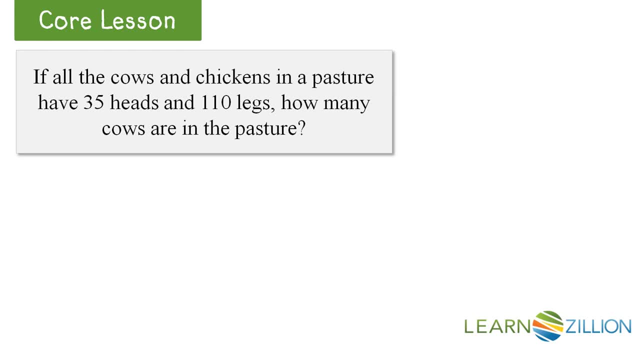 In step two we said that one equation would be about heads and the other would be about legs. Now let's take a closer look at the problem. We notice that all the cows and chickens have 35 heads. We know that every animal only has one head. so the number of cows, x plus the number of chickens, y. 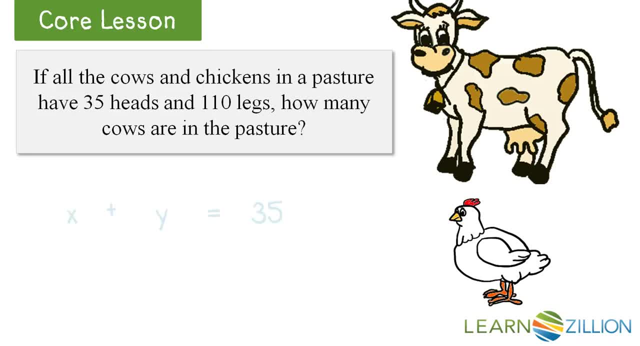 represents the total number of animal heads, 35, or x plus y equals 35.. This heads equation for our system is the number of cows and chickens, y, and the number of heads x plus y equals 35.. We also know that every cow has four legs, which means the total number of cows' legs is x times 4, or 4x. 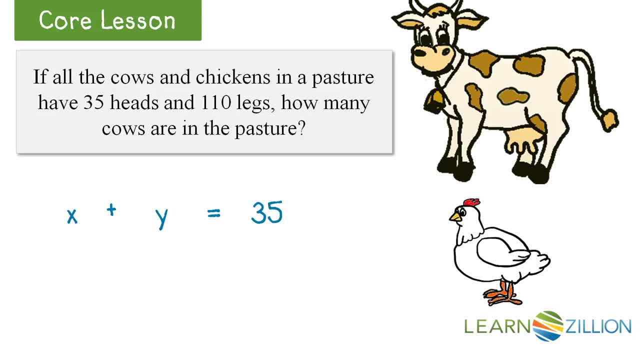 We know that each chicken has two legs, so the total number of chicken legs is 2 times y or 2y. The total number of animal legs in the pasture together is 110, so our legs equation is: 4x plus 2y equals 110. 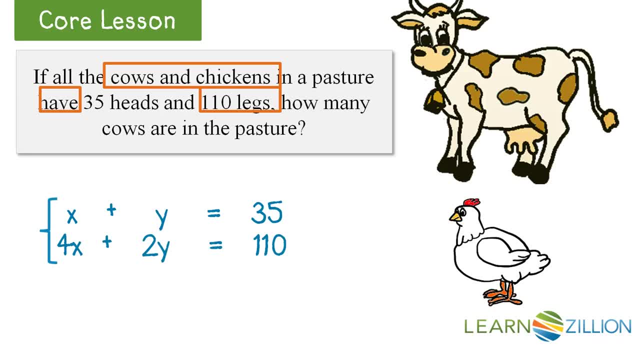 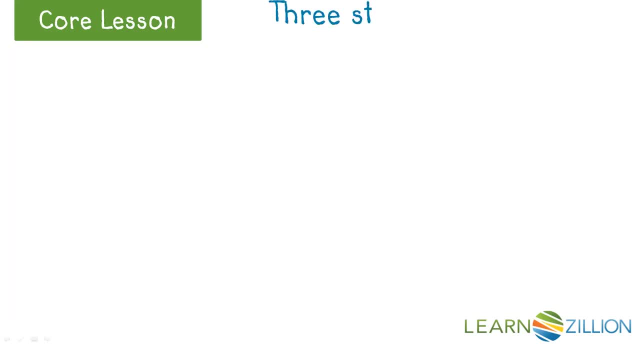 And here's our brace to say they're simultaneous equations, that the variables represent the same thing in both. and we've done it, We've written our system of equations. So the process has three steps. First, identify the unknowns and define your variables. 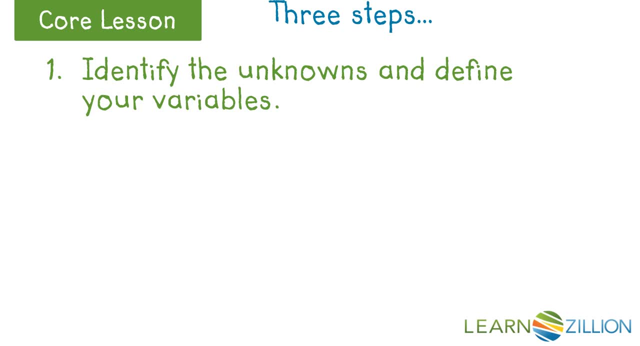 Remember, a system of equations has the same set of unknowns in all of its equations. Second, separate types of information. to know what the equations will describe, Be sure that one set of information represents a single thing about your unknowns and the other set of information represents a different thing about the unknowns.